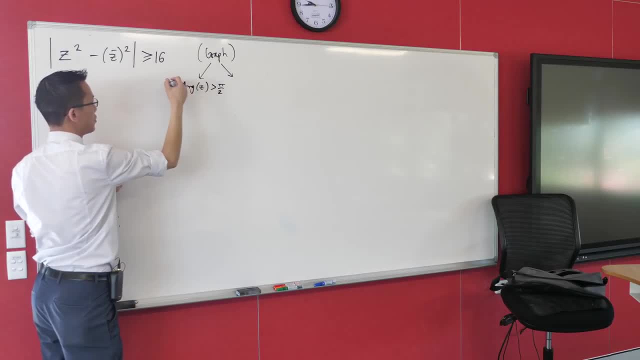 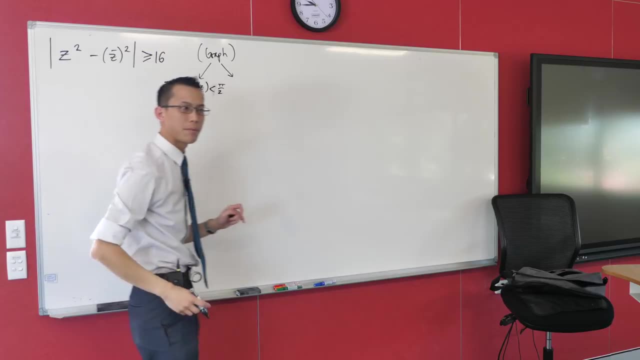 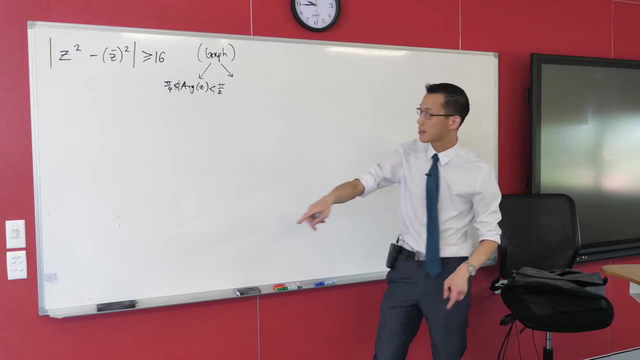 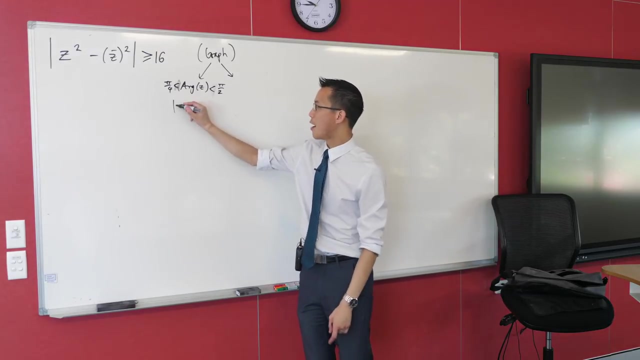 And you know, sorry, yeah, greater than pi over two. And I put my inequality the other way. let's make it less than and between pi over four, right? So you've got some complex number And when you measure its primary argument right from our positive real axis, it's going to be between pi over four and pi over two. So you know, there's that sector that you end up getting right. I could say: you know how about? mod z is just going to be less than three, Okay, so we're going to get what shape out of that. 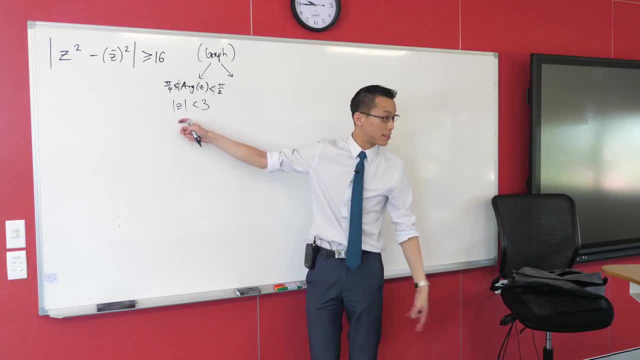 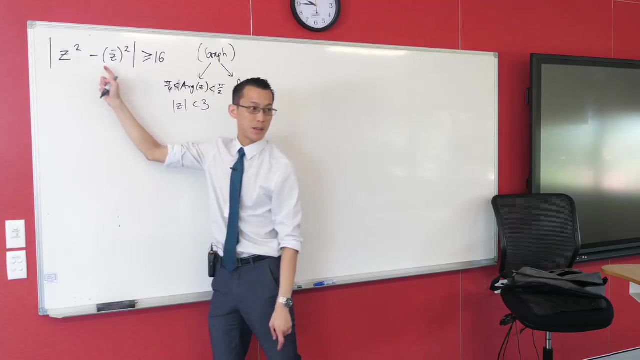 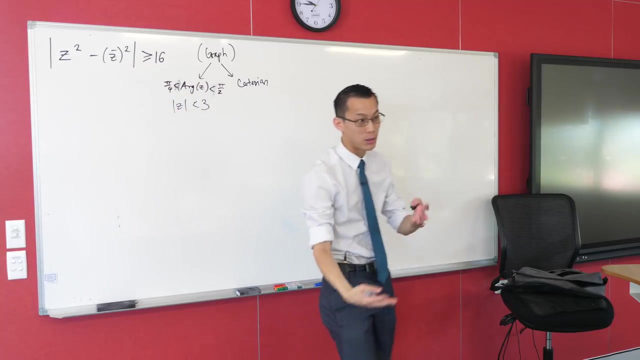 That's a circle, because we're just looking for the distance from the origin and make sure it's less than whatever is set right. So there's a whole bunch that you have to think of them in terms of just the complex numbers, But then there's those other kinds which essentially become a Cartesian graph. right, We're going to resolve these guys, because we're like I don't, I don't know what happens when you geometrically square the conjugate of a number and subtract that from like. I don't even know what that looks like in a ready way. I need to actually dig into the algebraic weeds and then try to find my way through there. 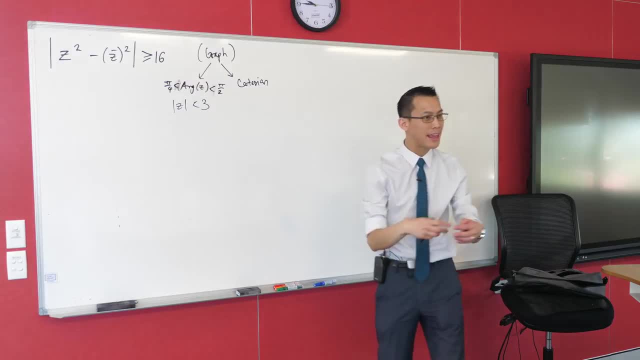 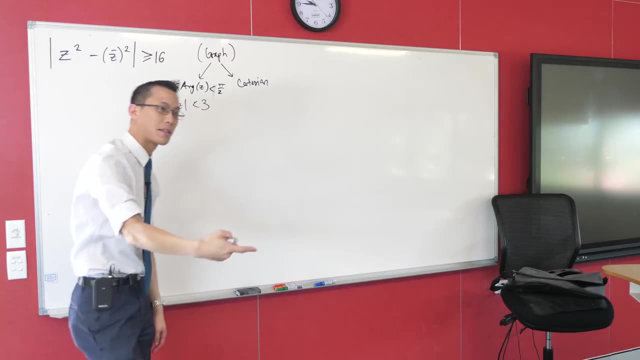 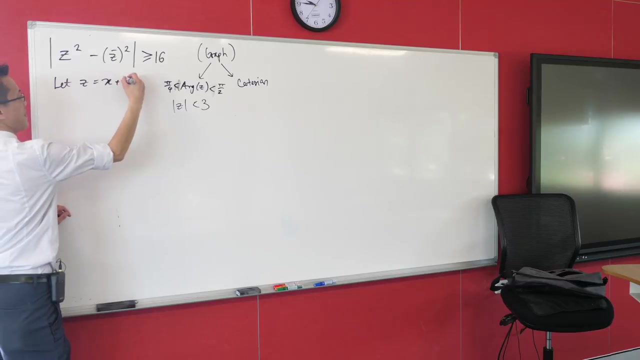 And get this in all x's and y's, Okay. so that's just to say, okay, we're cleaning, clearly leaning towards this family of functions. And so what are we going to do here? You actually need to state something right out the gate. Before you can even begin, you have to introduce some variables. right? What would you like to introduce? I'm going to start with: let z equal x plus i, y will be perfect, right? This is that Cartesian leaning. I mean, you could have said a plus ib, but then you're going to have an a axis and a b axis. 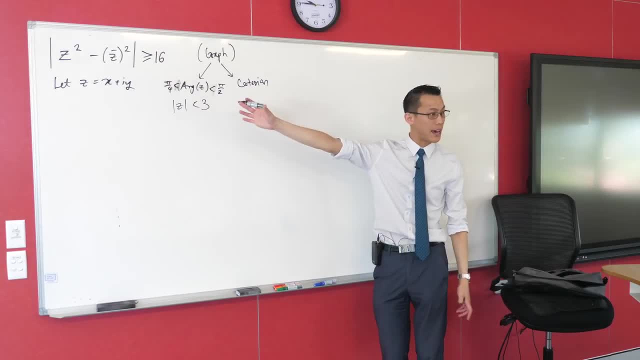 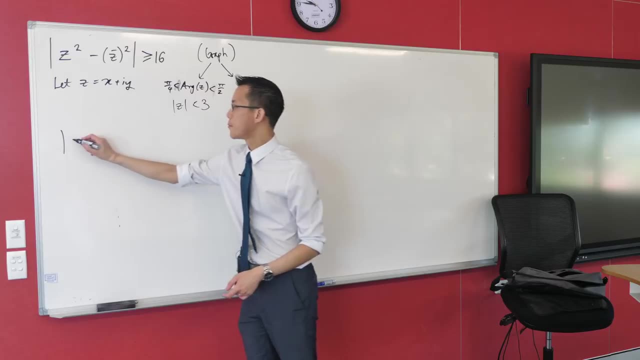 We just don't fit our brain as nice and neatly. So I'm going to introduce that, And that means that I can now express everything that I have here in terms of my x's and my y's. And I wonder how you went with this. I'm going to get my. I'm actually going to go straight to squaring it, because I think you know this well enough, right, If I've got my x plus i y in here and then I square, I'm going to get my x squared piece, I'm going to get my middle piece And then when I do my i y squared or i y squared, what am I going to get when I resolve that? 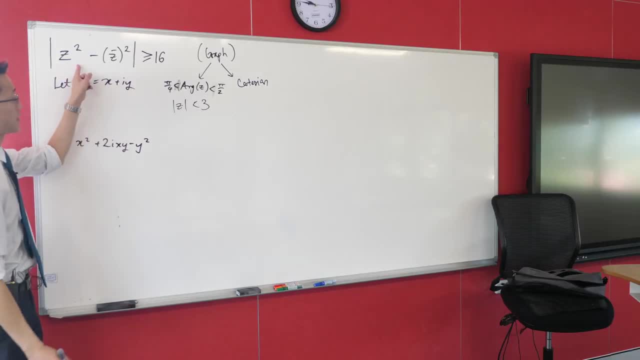 Minus y squared, Very good, Okay. So there's my expansion of just that number, And that's something which we want to become reasonably comfortable with doing. Then we're going to subtract. Okay, Now, because this is the conjugate right, We're doing all the same things. So is this x squared going to be any different? Nope, Same deal. 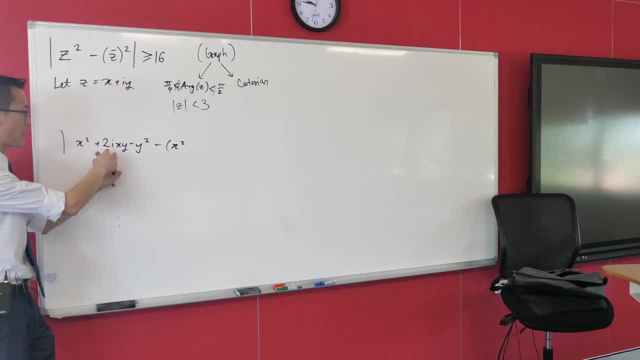 All right, this guy, how will this be different? Just a minus, because I'm going to have minus i y, multiplying in there Minus, What about this piece? Is this going to be plus? Hmm, Think, Think, Let's just. if whenever you're like, oh, now I'm not sure, then you go back. I mean, you don't want to waste time doing extra algebraic expansions that you don't need to, But if you do need to, then do it right. If I've got z bar x minus i y, let's do the squaring now. right, This whole thing gets squared. So I had my x squared, I had my minus 2xy, which you were happy with before. If you had a minus b, all squared, then this last piece right is going to be. 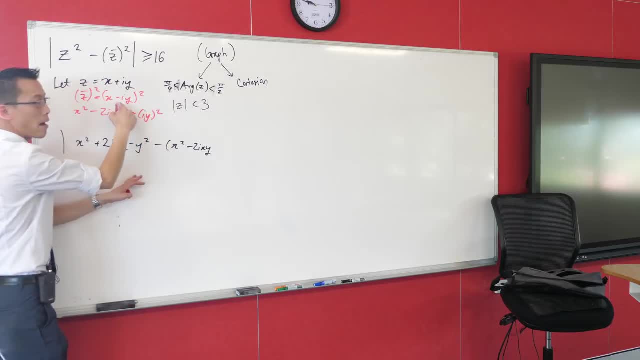 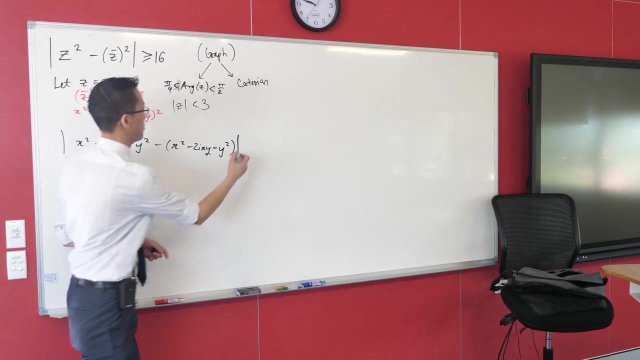 still plus i y squared, because the minus also gets squared, Is that okay? This minus that we had here came from the i's and that hasn't gone anywhere. So I'm still going to right Nope, wrong color, Minus y squared, Is that okay? And you can see clearly: a whole bunch of things are going to collapse here. That's why we like conjugates, because they fit so nicely together. Finish my modulus sign there and it's going to be greater than or equal to 16.. All right, Now, because we did it in this way, you can see the bit. 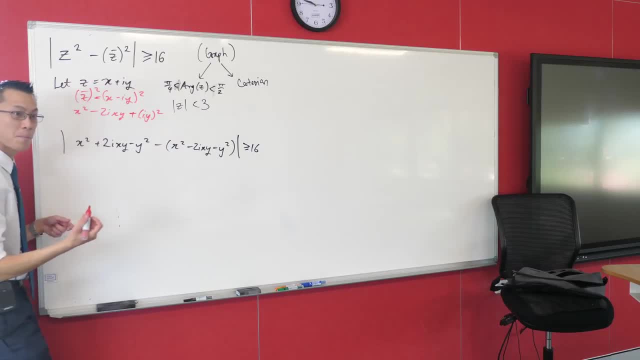 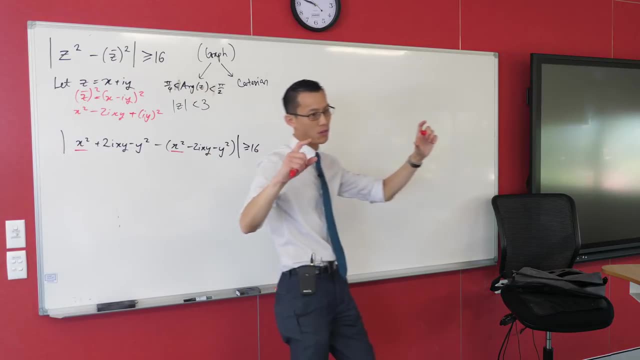 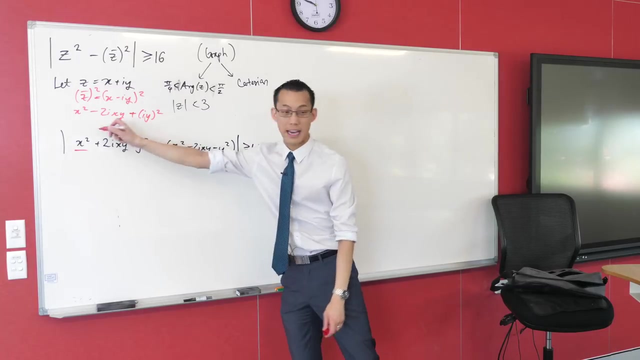 that are going to be nice and neat and going to fall out. Tell me what's going to cancel? First thing: Great, They're gone. By the way, I'm doing this very deliberately. When you've got a lot of terms to cancel, either by subtraction or by like, fractions and that kind of thing, I encourage you to do it like this. You know, if you've only got one other color with you, rather than like actually crossing out the thing, we look at your working right And it becomes harder to read, even if we know what you're doing. if you just like, scribble out things on top of it- So this does the same purpose, You can still see those are aligned. What else cancels? 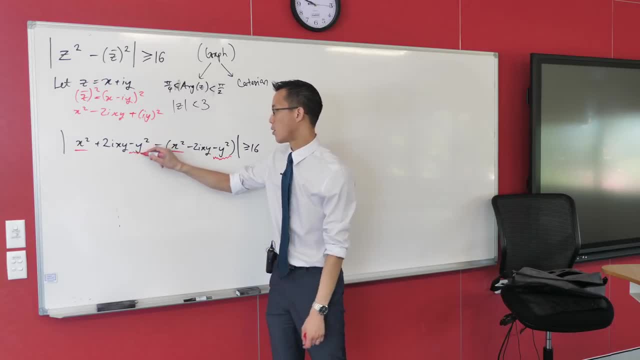 Yeah, So I've got a minus y squared there and a minus y squared there, And that's exactly how I'll write it, so that I can see the difference. Okay, So that's really good. That leaves me with: okay, what have I got here? Four ixy. Are you okay with that? Yep, Yes, Now I'm going to come to that i in a second. We'll deal with him briefly. I'm going to deal with my real numbers here, because they're nice and easy and they're positive as well. So I'm going to divide through by four ixy. 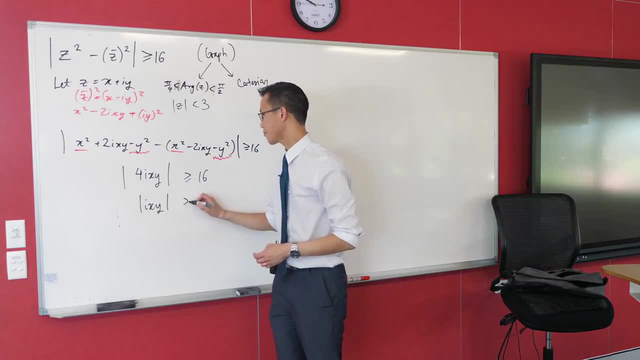 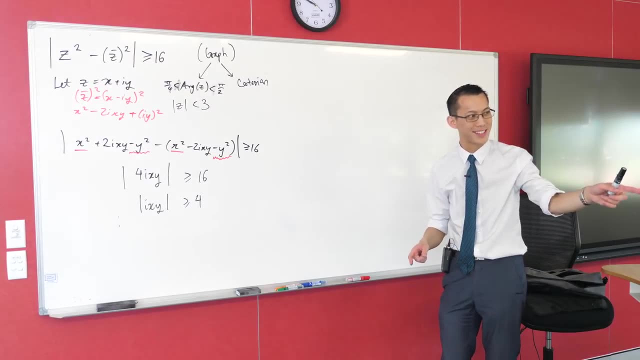 Four, which gives me this. And now I want you to pause, okay, Because seeing you got very close to this, but there's a subtle difference and I wonder if you've worked it out yet, because you're working so close but not quite. We need to think about this quite carefully. okay, If I gave you something like, say, the absolute value of five a, if we were just, you know, two unit students and we were living in real number land, we could really comfortably say: this is just five times the absolute value of a. 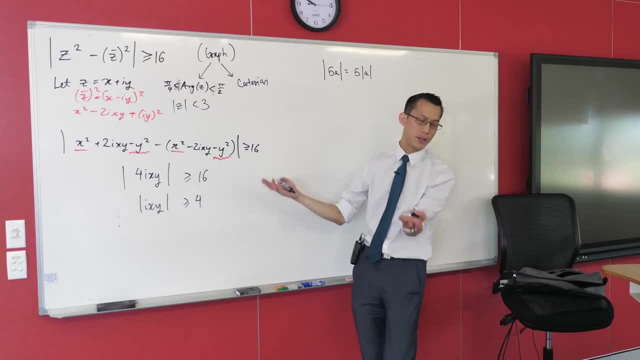 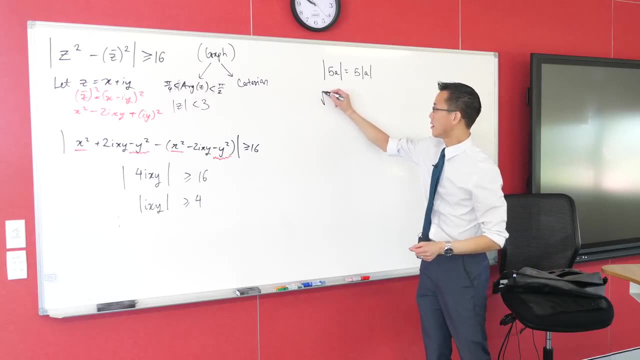 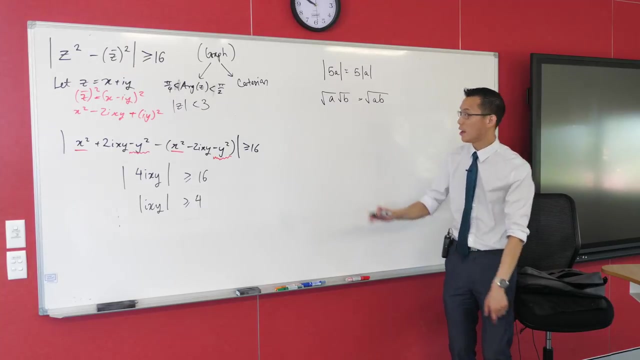 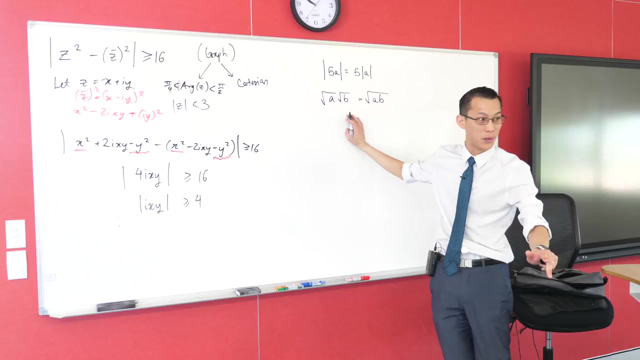 So that's kind of what we did here. when we divided through by four, We factorised out the four we divided through, we just did all in one hit. okay, But you have to be super careful dealing with complex numbers. You've already learned, hopefully you know this rule, This rule here that we've been using for ages with just normal real numbers. Are you guys familiar with what happens to this in complex number land? Have you encountered this before? If you haven't, tell me no, because then I'll explain it. But if you have, I don't want to bore you. So is it something you've met before? 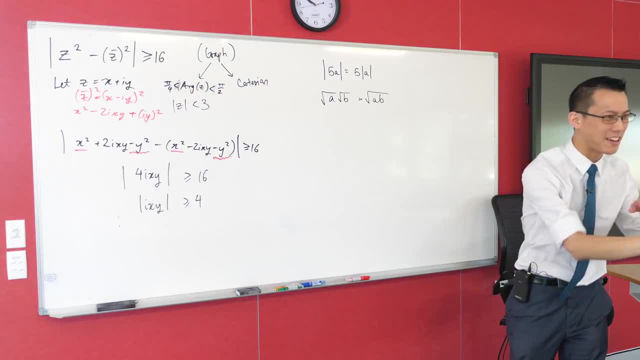 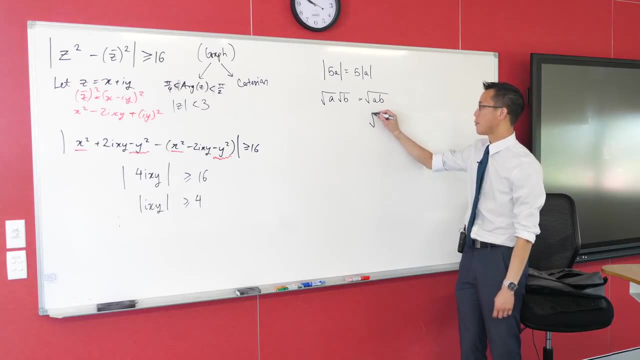 I saw your video on there. You got it from me. How about you guys? Has it been addressed in class? Okay? so let me just mention this. right, This is something we know what to do with. If, for example, I gave you the square root of 60, which is not square right, But we can see square numbers in there. So you guys should reflexively say: the biggest square that I can pull out of this is- I think it's going to be four- yeah. So you'd say, okay, that's the square root of four times the square root of 15, which gives you this right, And that's like a four. 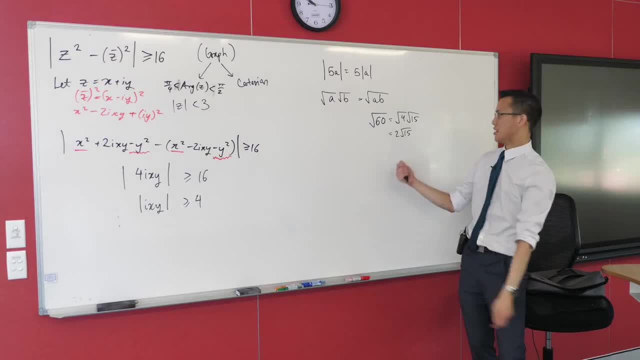 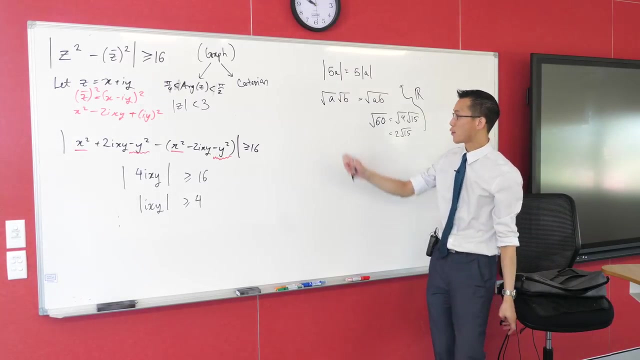 So that's like a big part of all we want you to do when we introduce thirds for the first time is do a whole bunch of simplifying, just like this: okay, This is fine, this is fine in real numbers. okay, Everything looks happy there. But essentially the second you enter the complex set, you run into troubles. For example, what happens if both a and b are just negative one? okay, 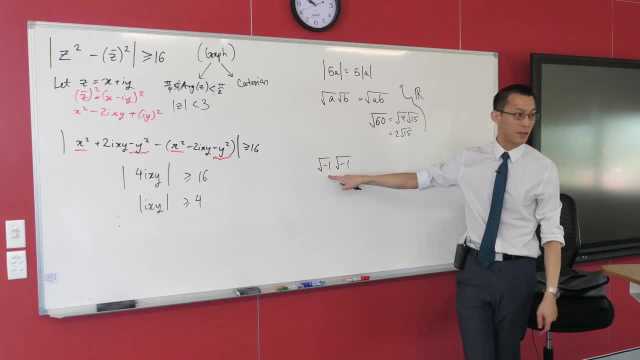 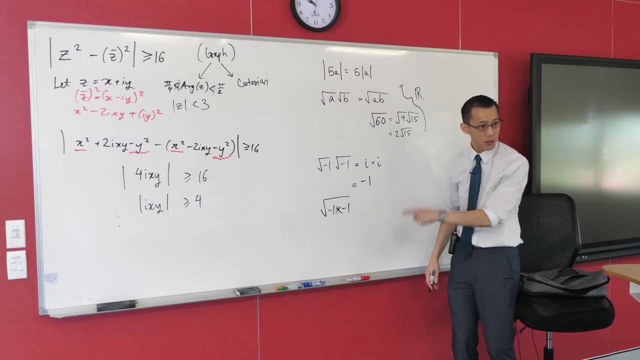 Now if we're in complex number land, right, We have a name for negative, for the square root of 60.. The square root of negative one, we call it. It is the basic building block, right? So you should be able to tell me we just did, i squared over there. The answer, of course, is minus one. okay, But if I use this rule, which you've relied on very faithfully for many years now, and see what happens if I try and draw an equality here- Sorry, it's a really bad multiplication time- That's better. Have you noticed what happens? right? This is my square root of ab. Negative one times negative one, of course, is just one. 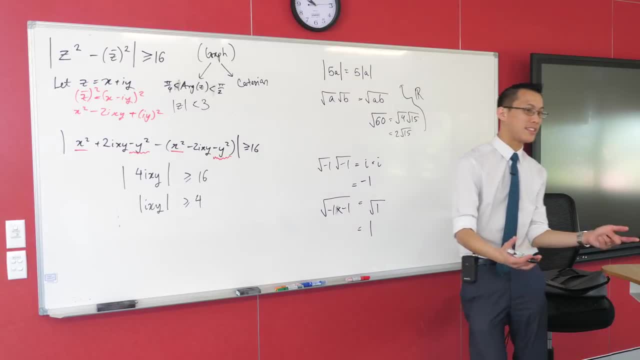 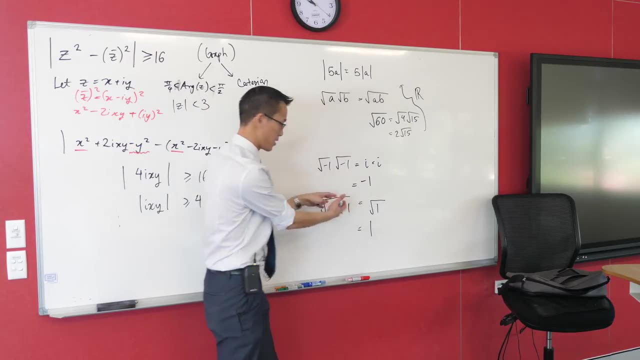 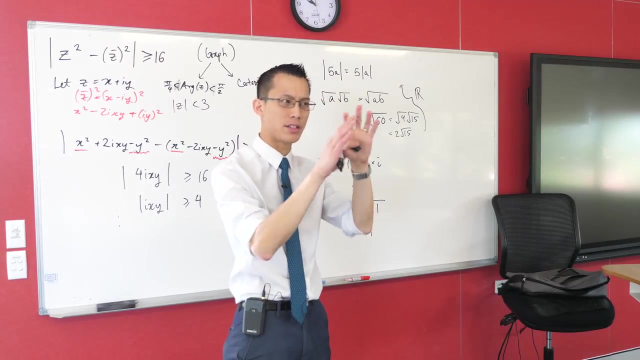 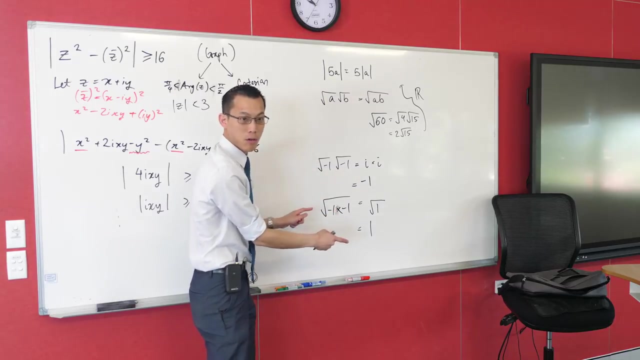 You're like uh-oh, Okay, What happened? And the answer is: this rule actually only works when a and b are both strictly positive. If we are willing to deal with complex numbers suddenly, things break down. By the way, just for extra bonus points, I think it's probably not until you haven't done inverse functions as a topic yet, have you? No, not yet. You will encounter that next year, so that you can do inverse trig and what have you. And part of the reason why this is a problem is because the square root function- right, It's an inverse function with a restricted domain. 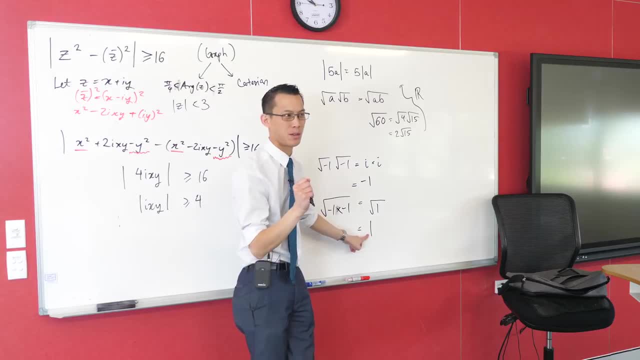 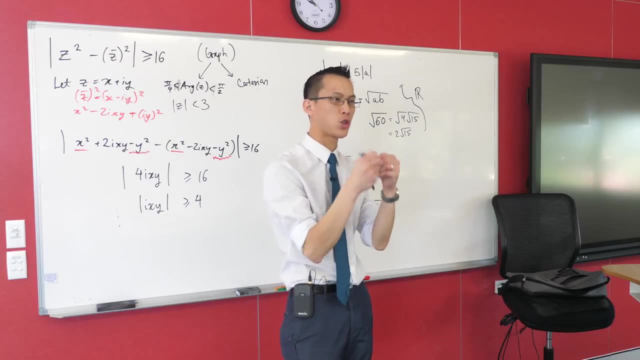 Why do we restrict it to the positives? Quick question for you: Why do we restrict it to the positives? Why don't we let like? give me a word definition, a verbal definition of the square root of something is: How would you define that? 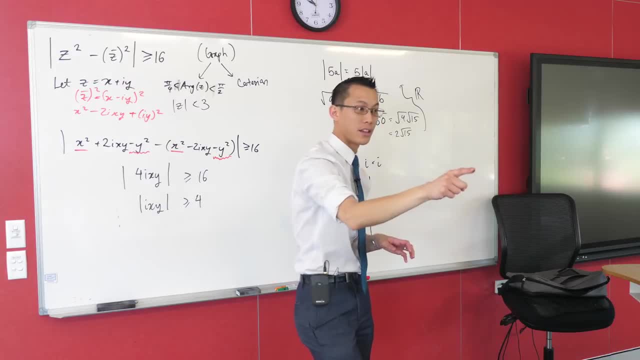 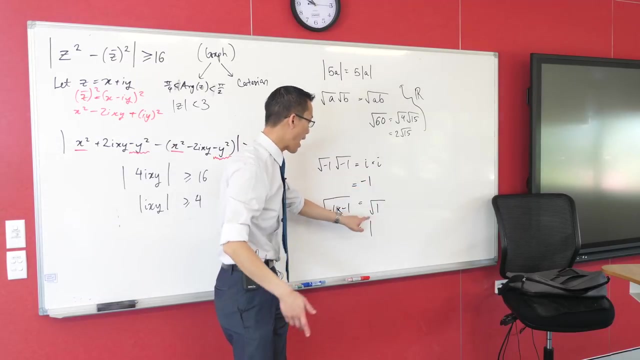 Hmm, Yep, Yeah. Let me say that again. See if I got that right and see if you guys agree: The square root of something is the number, that if you multiply it by itself, you'll get your number right. This isn't negative one by that definition- one of the square roots of one, because if you multiply this by itself, sure enough you get there right.